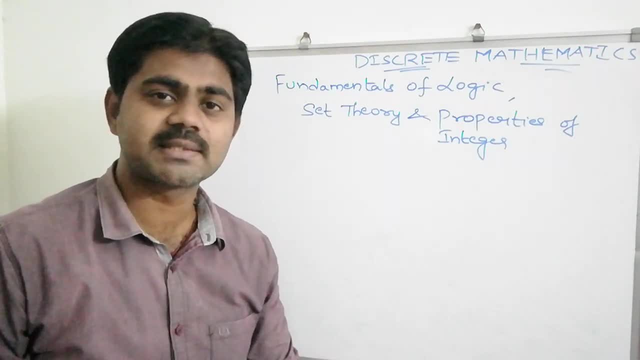 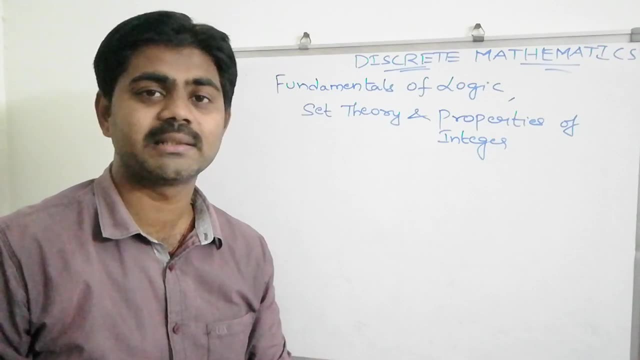 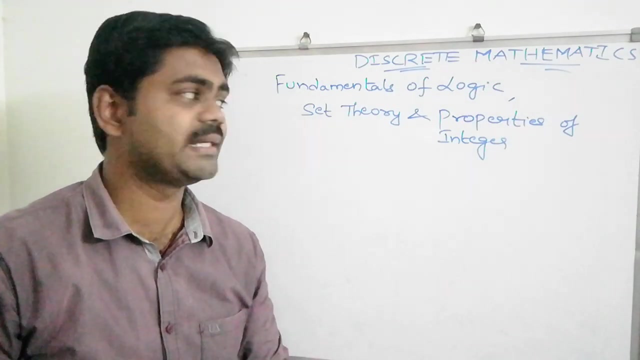 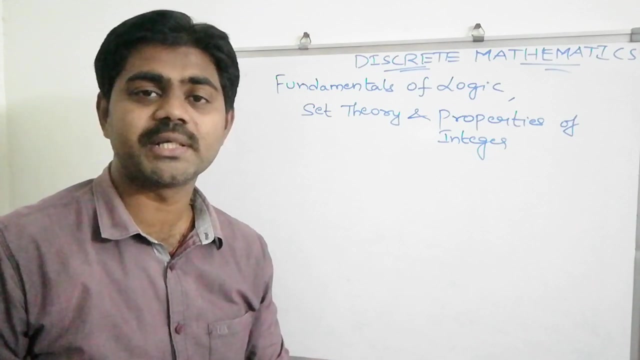 And properties of integer. So, anyways, we already studied this set theory in our intermediate or 10th class, like that. But anyhow, first we'll know the basics of fundamentals of logic, set theory and properties of integer. So before going to that, first we should know statements and notations. So what is statement and how we'll have a notation for that statement. 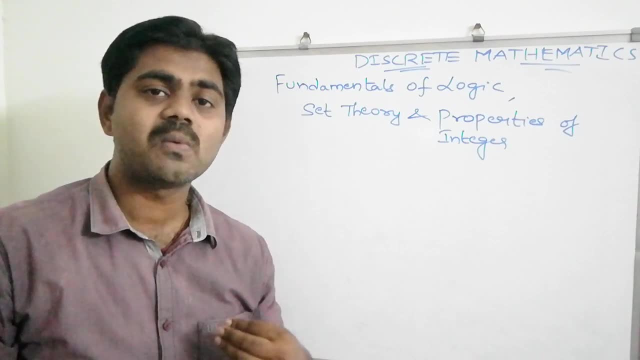 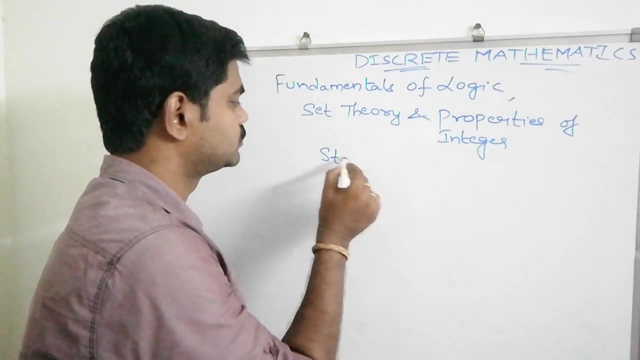 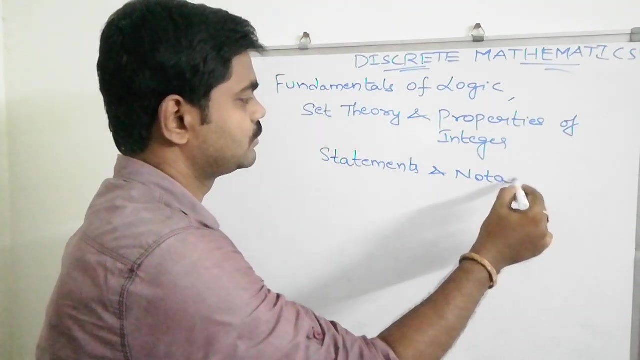 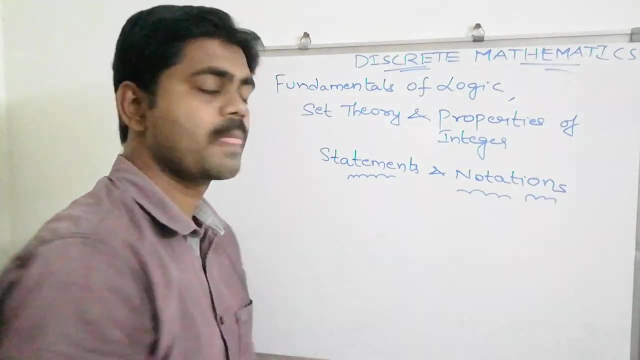 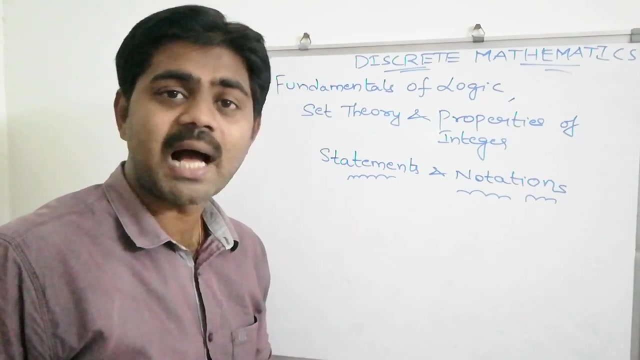 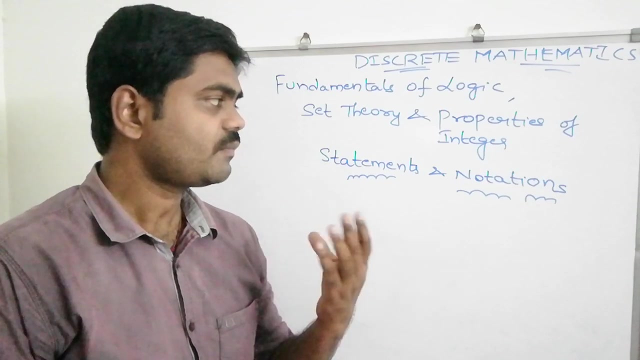 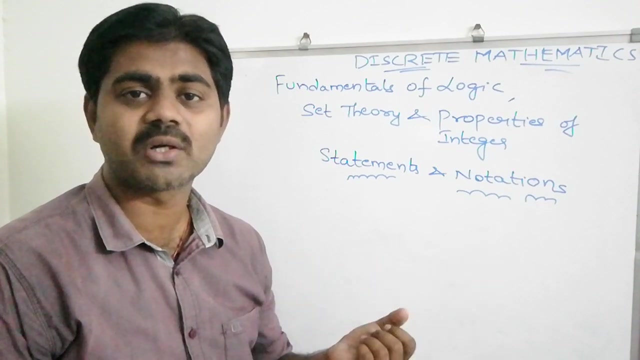 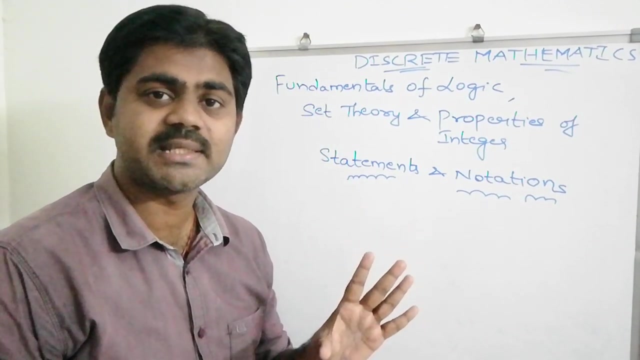 For example, if I say English statement, how I need to project that English statement in more logical way. Okay, Okay. statements and notations: Okay. so in symbolic logic we'll study arguments. So depending upon the arguments, we'll have logical statements And depending upon the English statement and the words, we can clearly say whether it is a statement or not. For example, let us see some examples. These are clear statements And after that we'll see how we have a notation for those statements. So let us see some examples of statements. 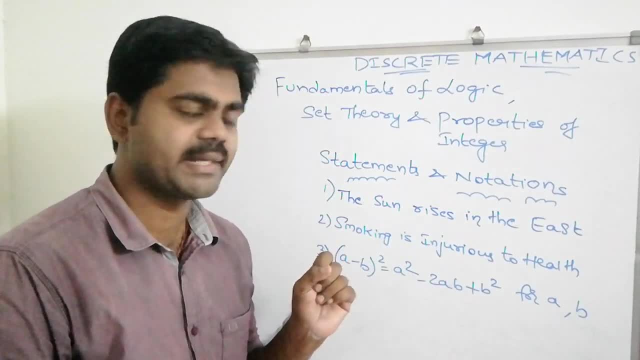 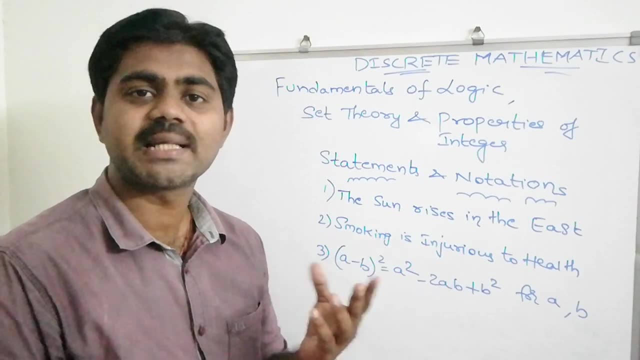 Okay. so if we see the statements here, the Sun rises in the east. The most important thing which we need to focus upon is the truth. Okay, we know that the Sun rises in the east, isn't it? It is true, It is a statement. Smoking is injurious to health. Is it true or not? Yes, smoking is harm to our health or injurious to health. This is also true. And A minus b- whole square equal to a squared minus two: A squared minus two. A squared minus two equal to b squared. This is correct. The sun is rising in the east and it is an injurious to health. 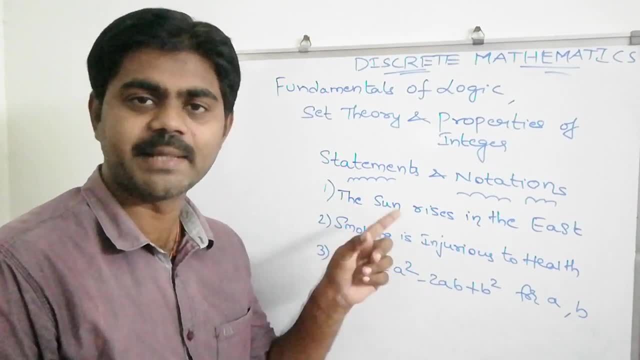 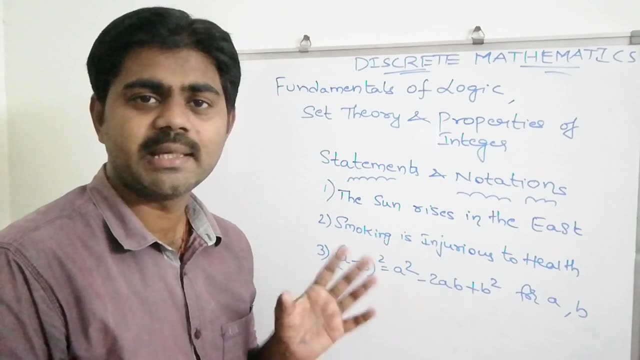 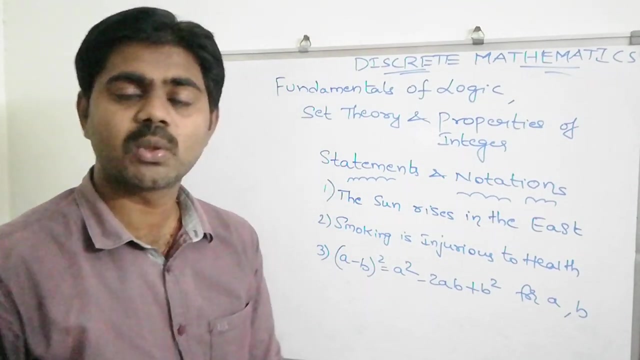 in the East, isn't it? it is true, it is a statement. smoking is injurious to health. is it true or not? yes, smoking is harm to health or injurious to health. this is also true. and a minus B- whole square equal to a square minus 2. a B plus B. 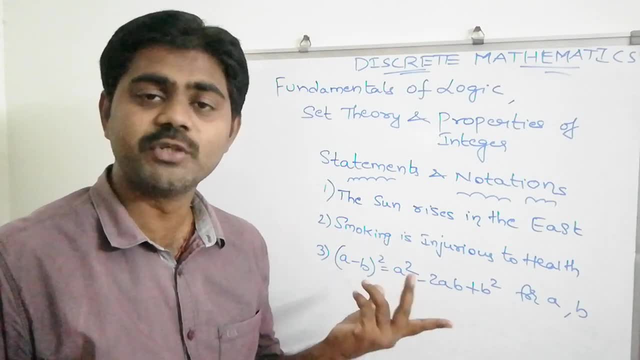 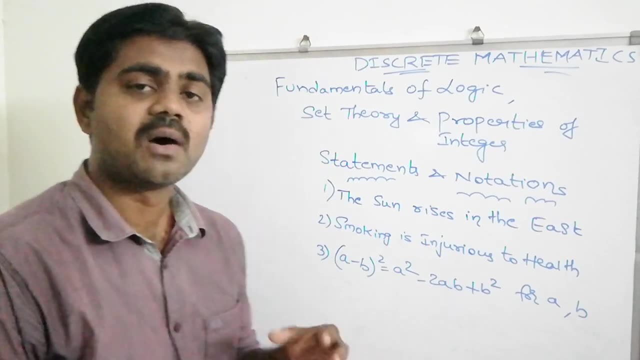 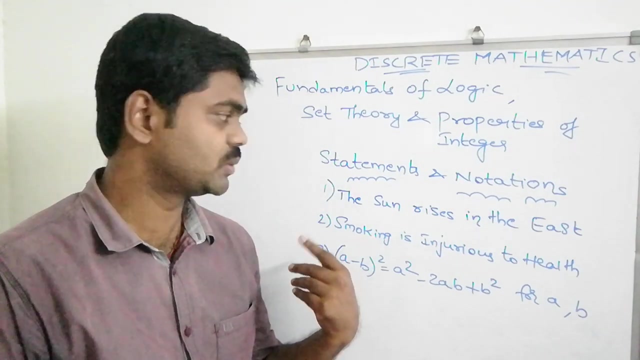 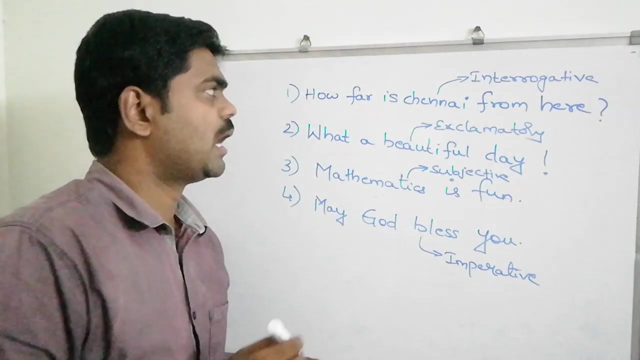 square for a and B. even this is a universal truth. these are all statements. so I can clearly say these three are statement. what all are not statements? we'll see some examples of the English words or sentences were not statements. let us see some examples for that. so if you see here how far is 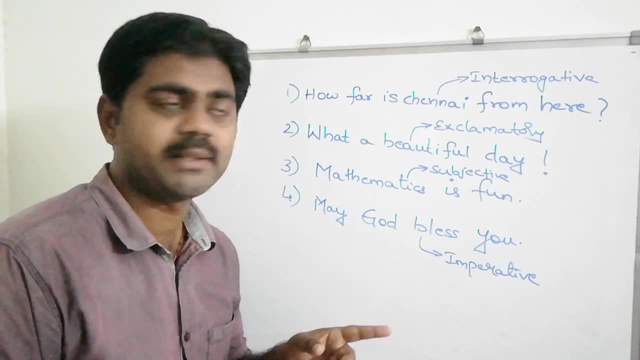 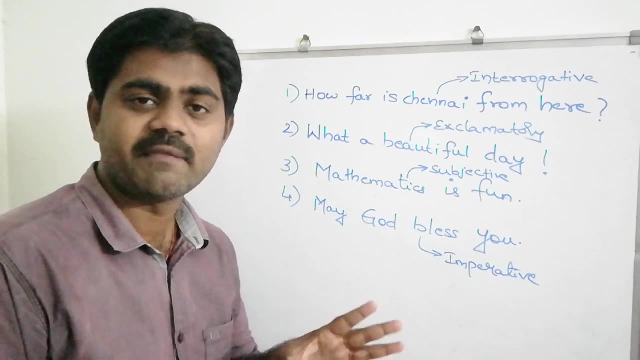 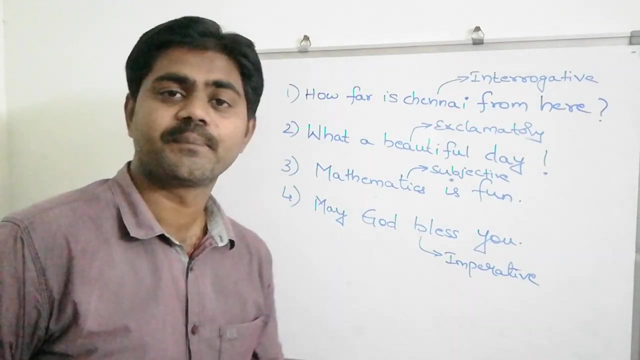 charnai from here. it's a question mark, right, so it is an interrogative statement. remember: when can a sentence be a statement? whenever a sentence can be a statement, it is declarative. That means either true or false. How far is Chennai from here? That? 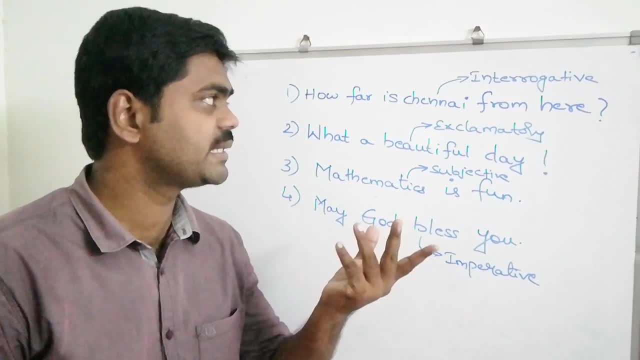 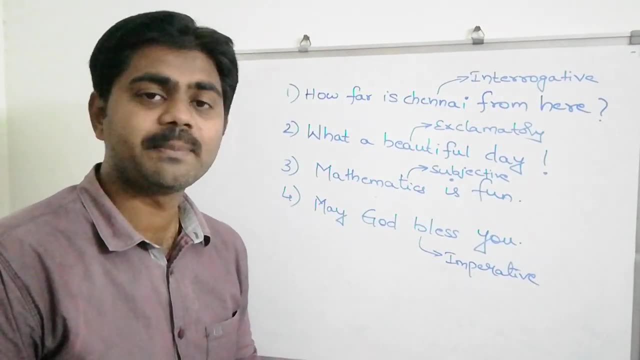 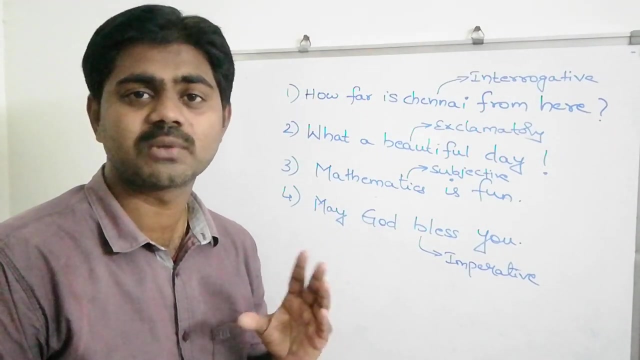 means we are asking a question that how far is Chennai from here? It's an interrogative, so it is not a statement. Second one: What a beautiful day. It's exclamatory mark, Right, So this is also not a statement. Third one: Mathematics is fun And this one is subjective. 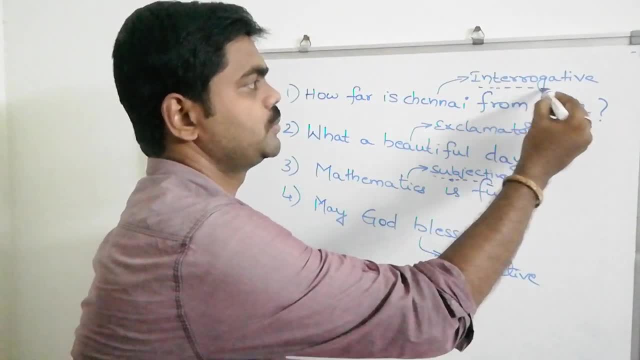 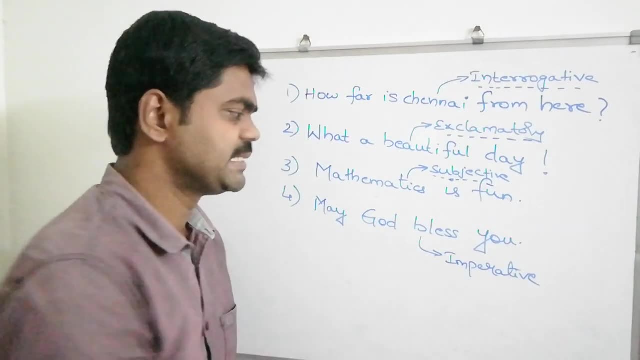 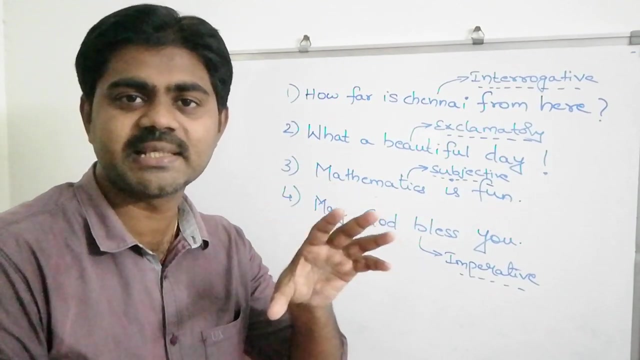 The first one is interrogative, Second one is exclamatory, Third one is subjective And fourth one- may God bless you. This is imperative. So all these are not statements. Remember if any English words or any English sentences will become statements only when they are. 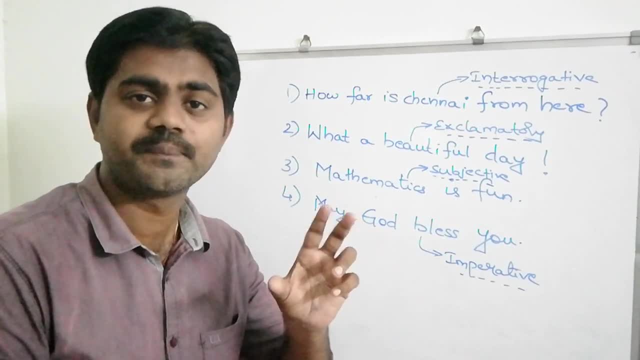 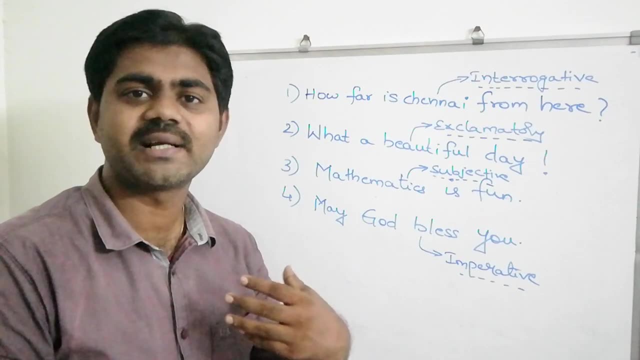 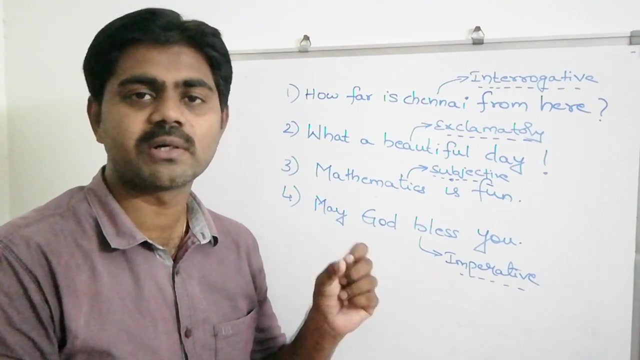 declarative Right. So declarative in the sense. is it true or false? I hope you understood. So these are all not statements. So we came to know that what are different statements, How we will write statements. Now let us have a notation for each and every statement. So why? because 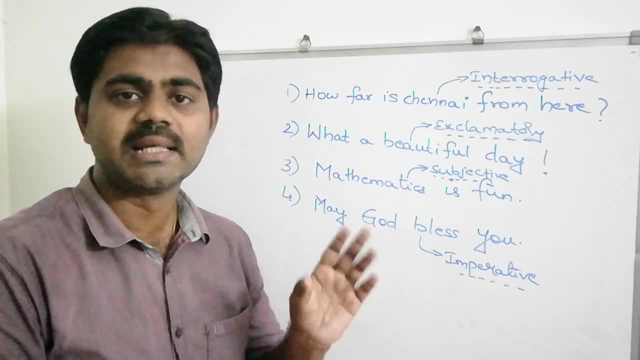 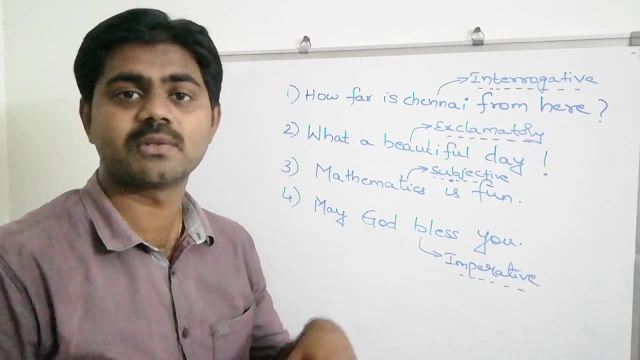 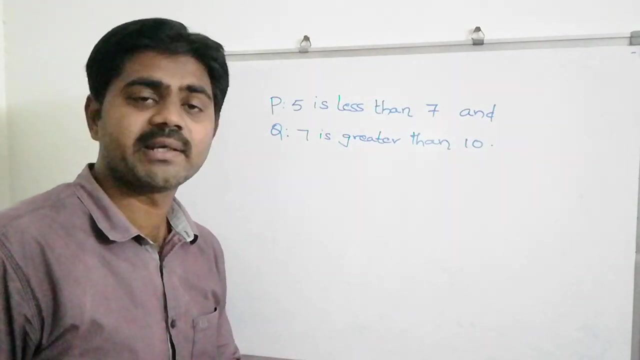 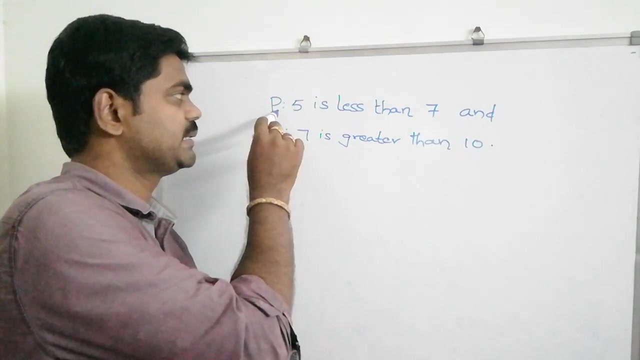 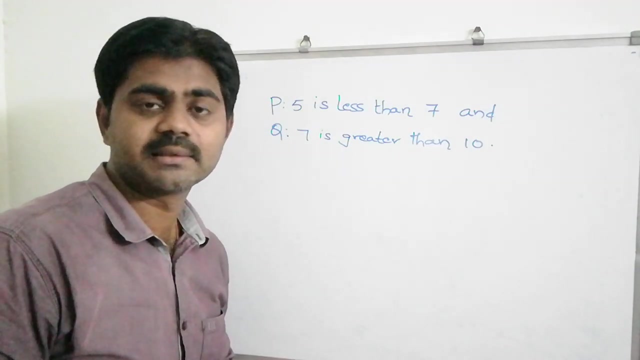 our topic is statements and notations. Let's see how we denote our statements into notations. So if you see an example here, 5 is less than 7. So I denoted in p, So I took a variable p colon: 5 is less than 7 and q, 7 is greater than 10.. So I can clearly say these two are: 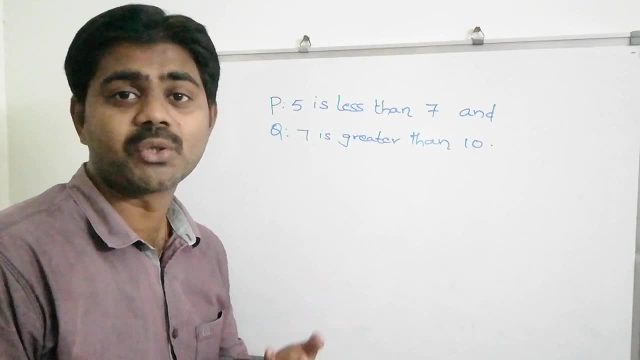 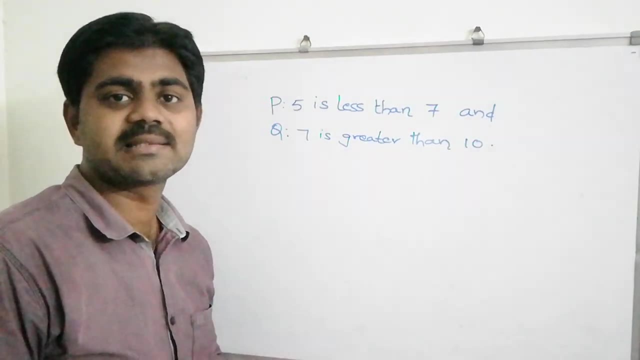 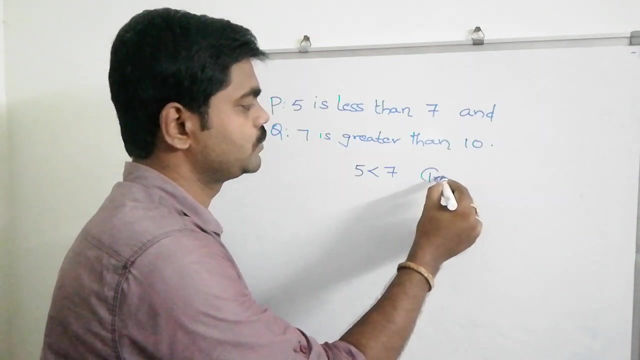 statements. Why? Because these two are declarative, Either true or false. So which one is true and which one is holding false? If you clearly see, p 5 is less than 7.. As we know that 5 is always less than 7.. This is true. So p is true. So what about second one here? 7 is. 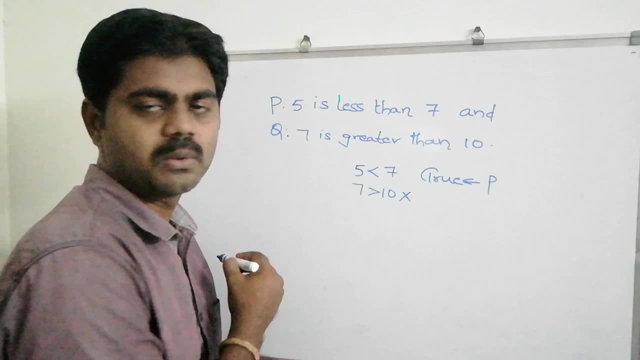 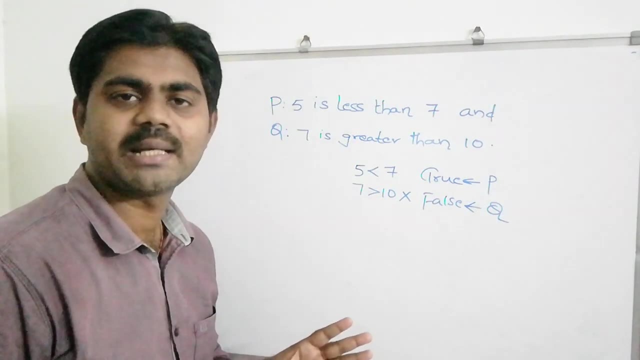 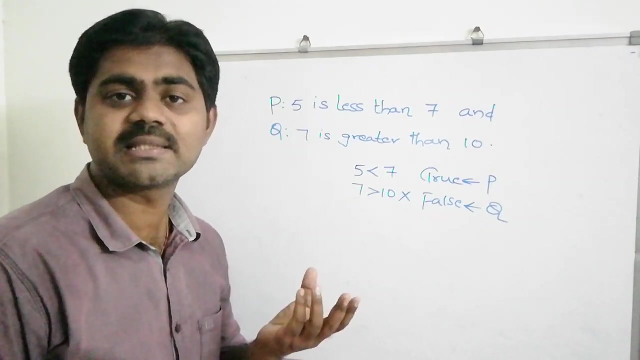 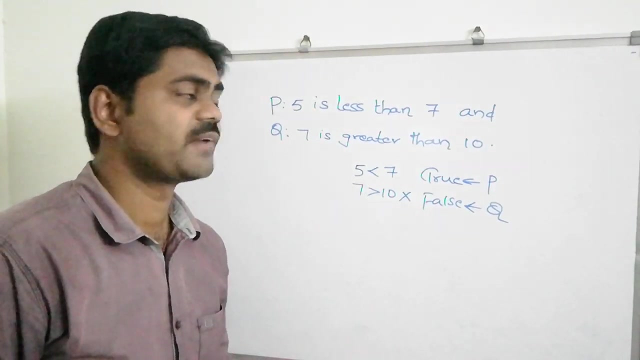 greater than 10.. Isn't it No, False? So q is false, Then these both can be statements, Right? So once we know the notation of different statements, then we can have connectives. So what are connectives here? For example, if I say 5 is less than 7 and I also need 7, is 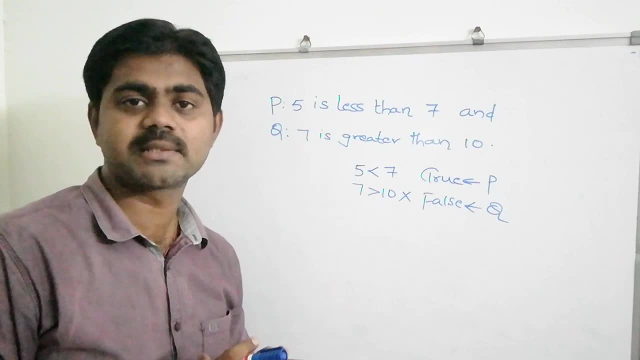 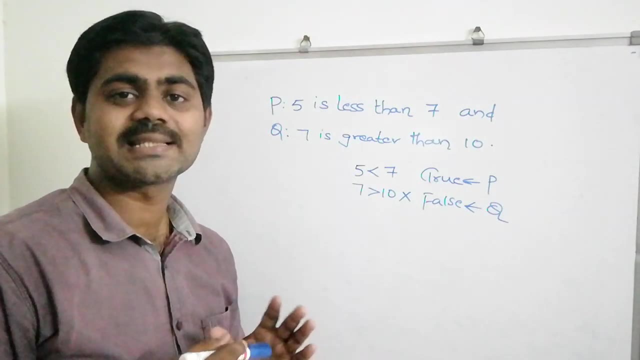 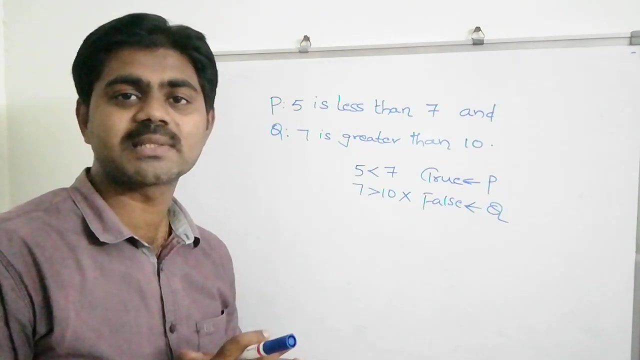 greater than 10.. Then I am connecting these two statements: 5 is less than 7, under 7 is greater than 10.. So I should need some connectives. So let us see what are the basic connectives and how we denote those connectives and how we construct truth tables. So truth tables. 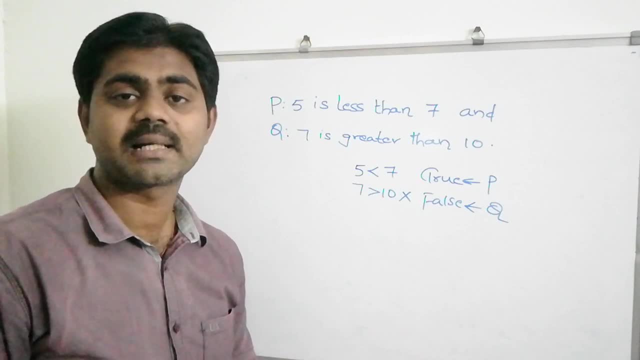 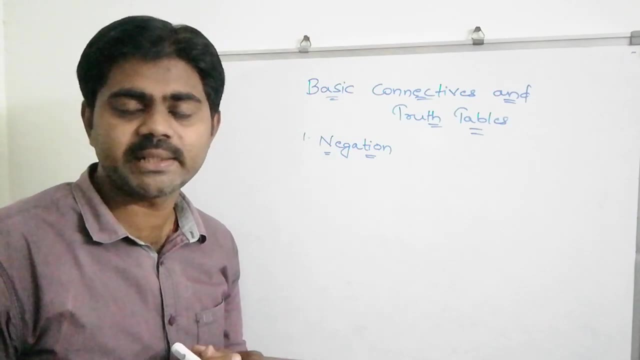 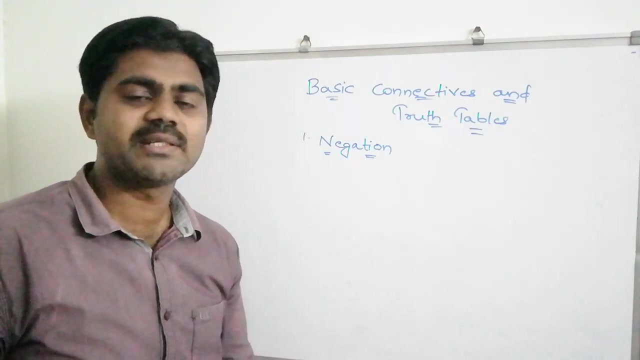 plays a major role here. Okay, So let us see some connectives. See, in order to connect two statements, I require connectives, Right? So in that? first I will discuss about negation. Okay, So negation is basically applicable for any single statement. 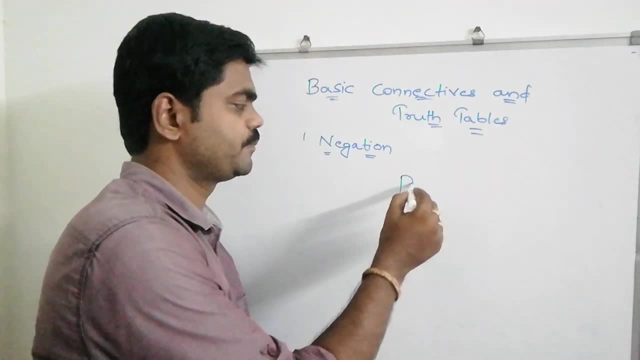 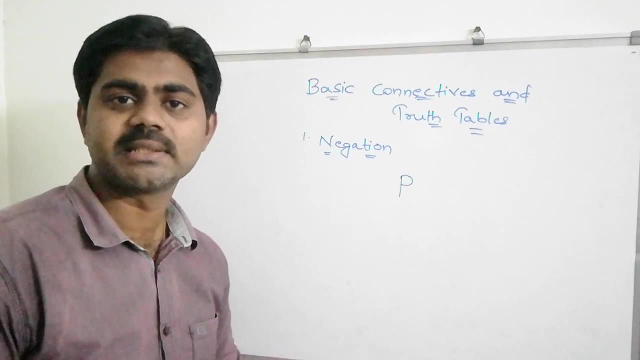 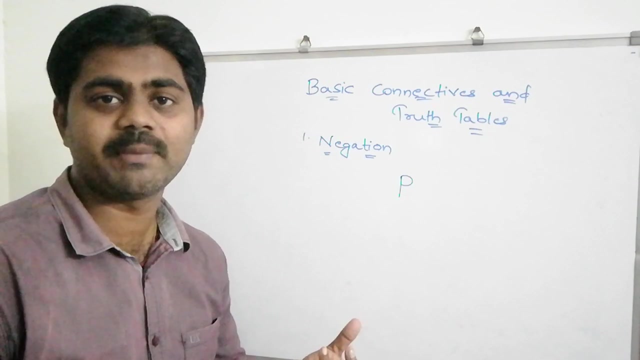 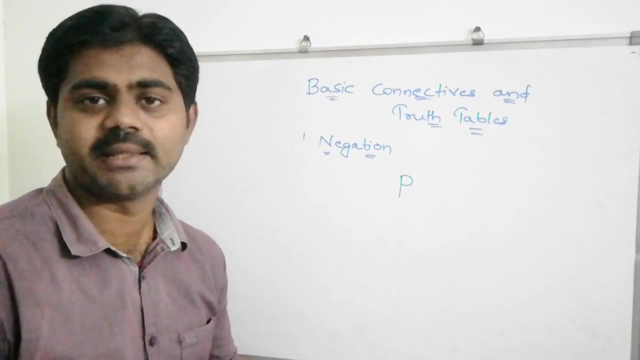 For example, if I have p, then I can have negation of p. So what is negation here? Not Exactly opposite? So if I say it rains today, So what is negation of that statement p, It will not rain today? Okay, For example, today is Sunday. What is negation for that statement Today? 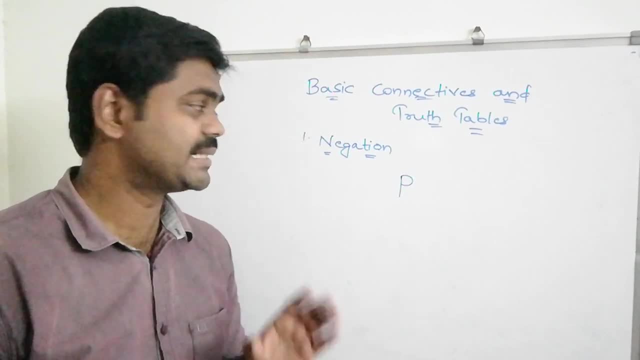 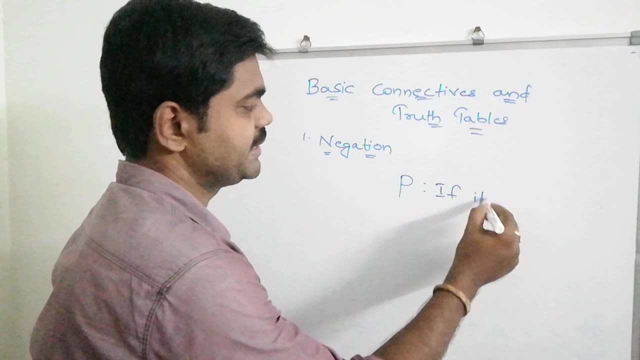 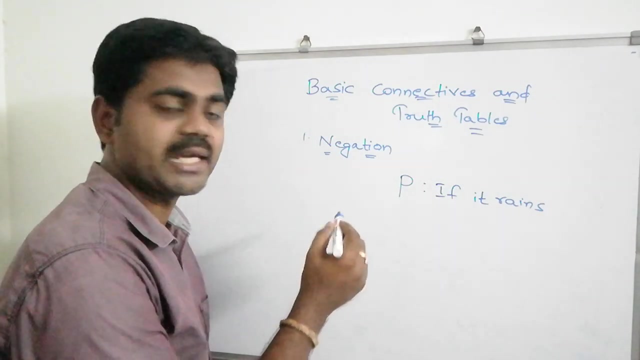 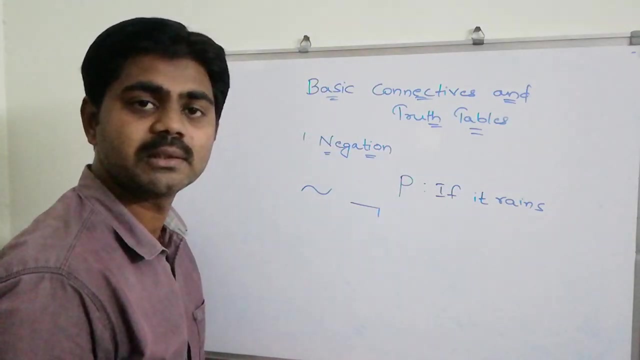 is not Sunday, Okay. So negation is not Okay. So for statement, if it rains. So how your negation is denoted. So the symbol for negation is tilt symbol or this one or this one. So we have three symbols. We can use any symbol here. 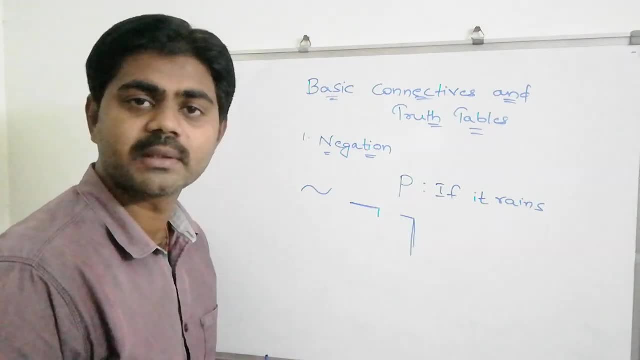 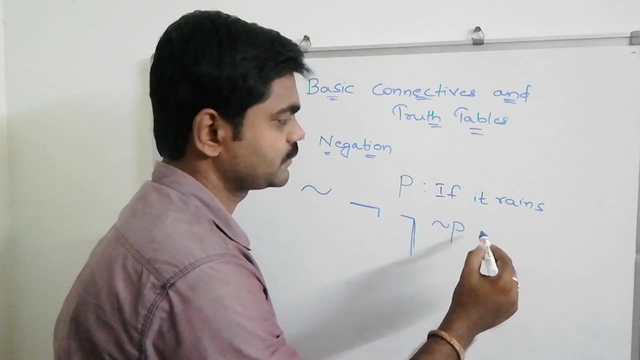 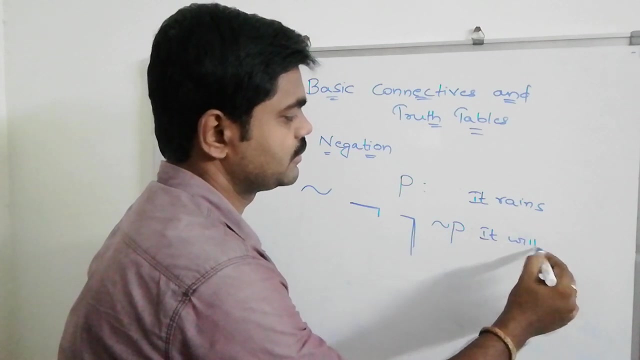 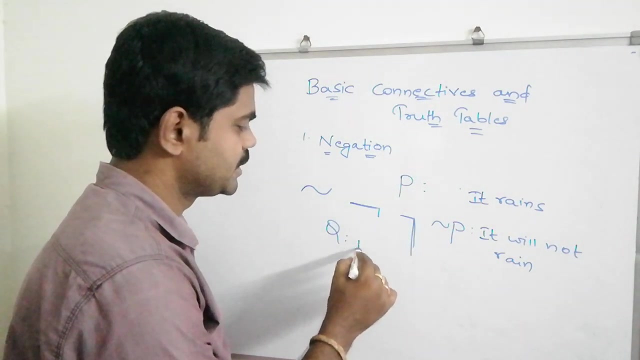 This one or this one. So if I say p, if it rains, If I say like this negation: p, Sorry It rains, It will not rain. So if I take another statement, q, Today is Sunday, Okay, So if I 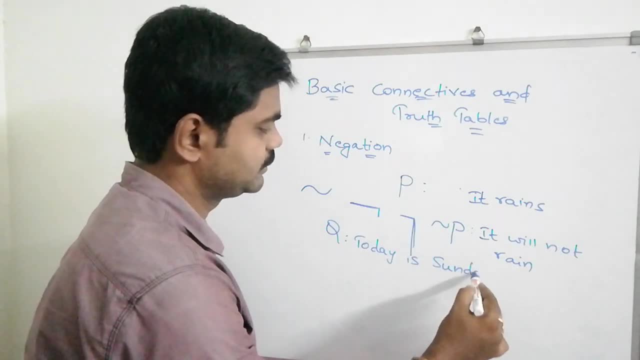 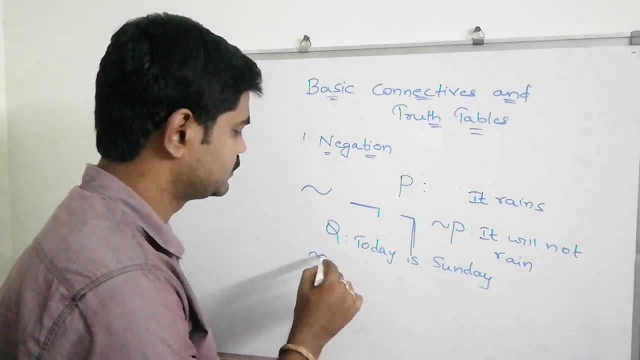 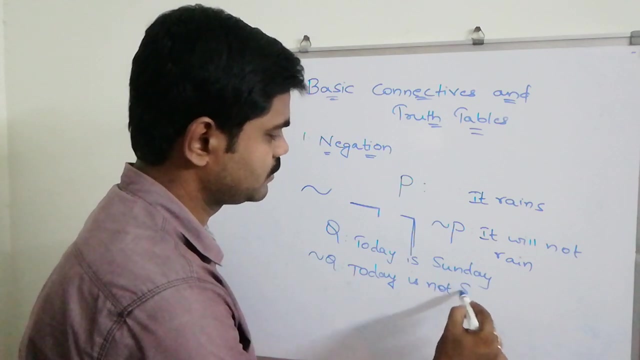 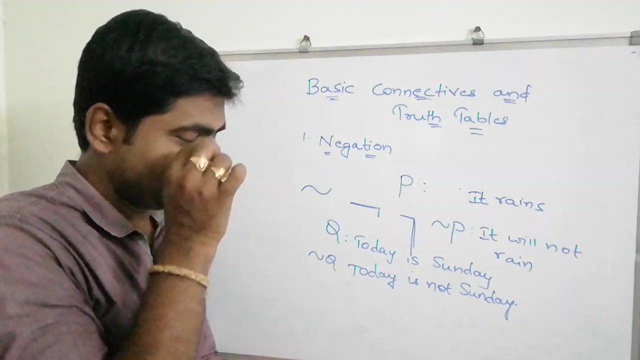 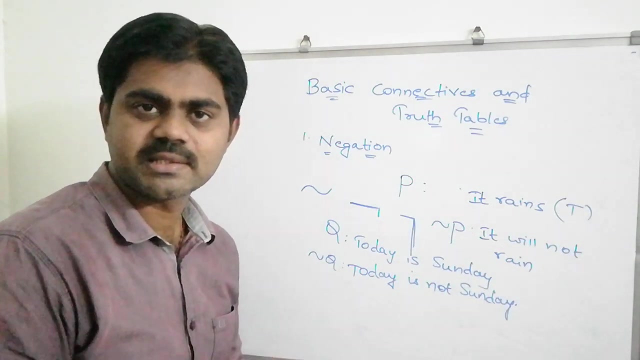 say: today is Sunday, Okay. So what is negation of q? Today is not Sunday Like that, Okay. So if this one is true, Okay. So the first one is p. So the negation of that one is false If the first one is false. 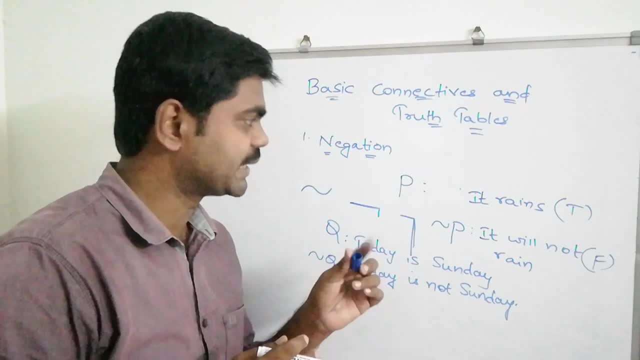 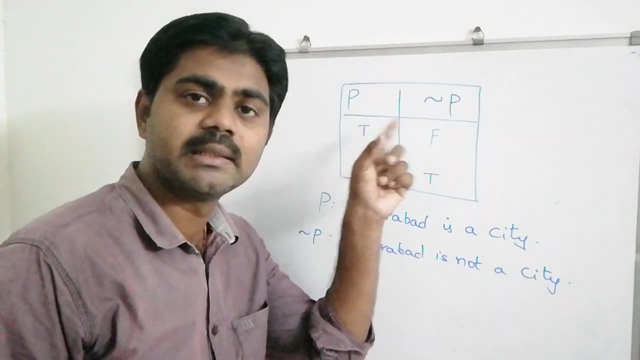 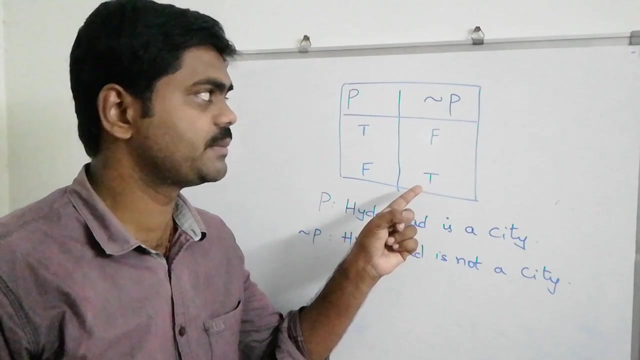 then negation of that one is true. So now we construct a truth table for this. So let us see truth table for this. I have p and negation p. If p is true, negation p is false. If p is false, negation p is true. So there is no rule that negation can be applied only. 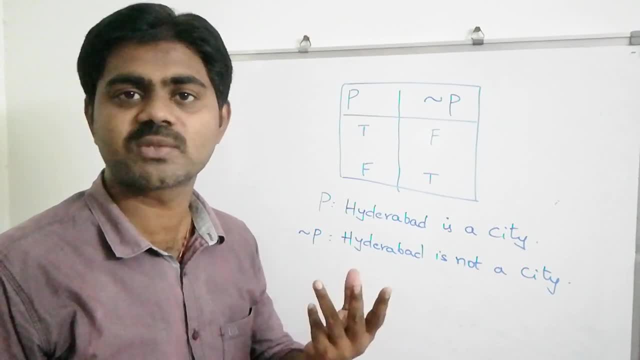 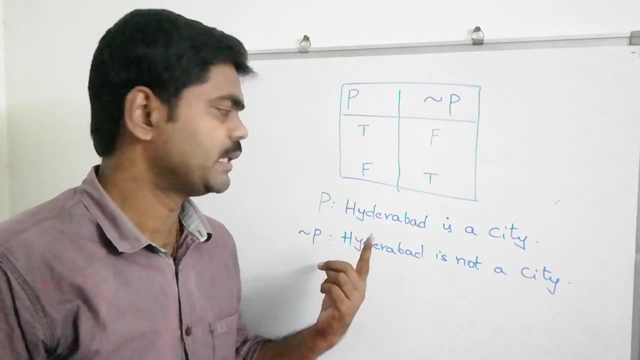 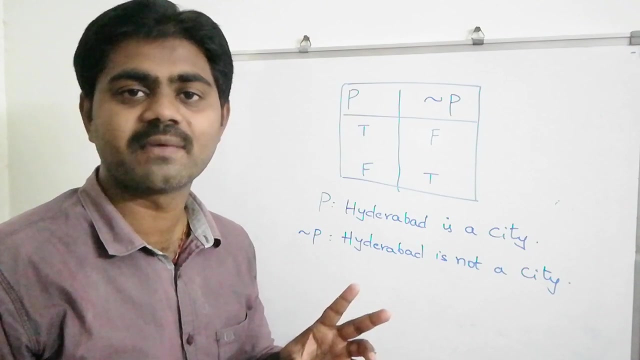 p, You can apply on Q, you can apply on R, you can apply on S, whatever. So, in English statement, if you see P, if Hyderabad is a city, what about negation P? Hyderabad is not a city. So this is the first connective and second one. 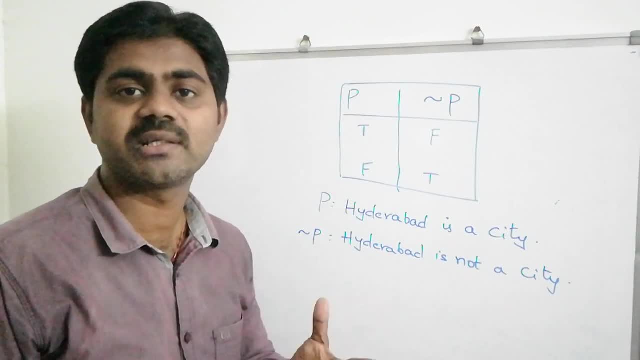 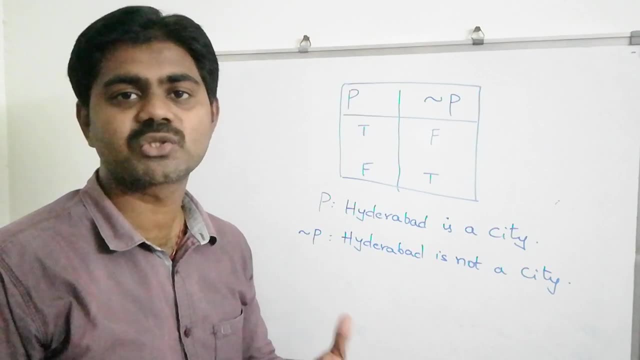 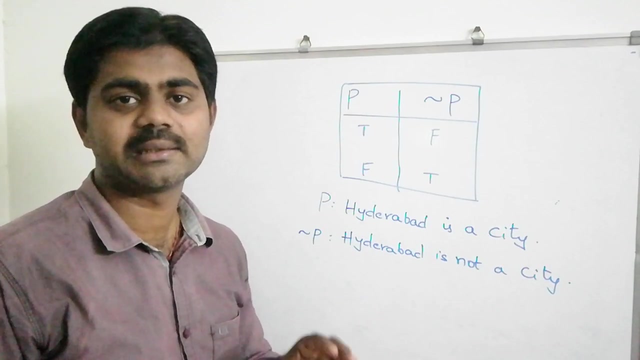 So second one is conjunction. So what is conjunction here? And So I need both. So okay, for example, if it rains today, then So if then is entirely different. So what is conjunction here? A connective which connects two statements. 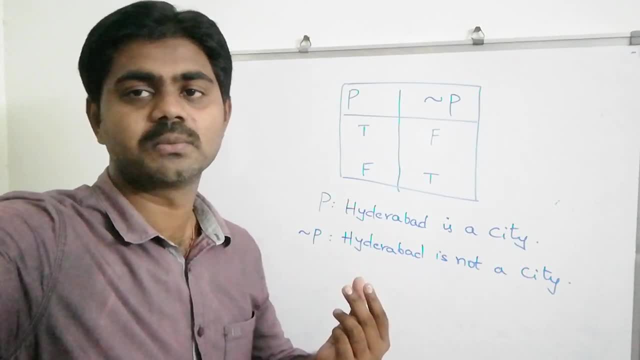 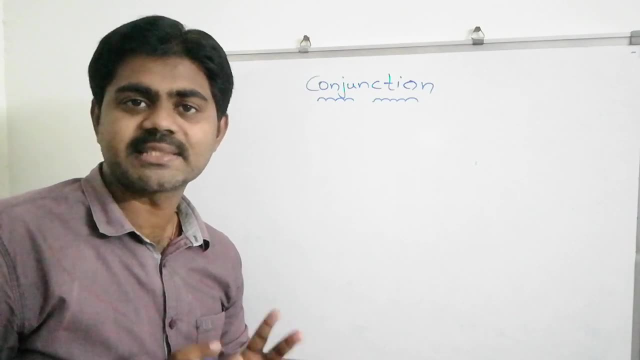 So it's basically, and So let us see connective. So the next one is conjunction. So what is conjunction here? And So if we have two statements, P and Q, then I will use conjunction to combine, Combine these two. 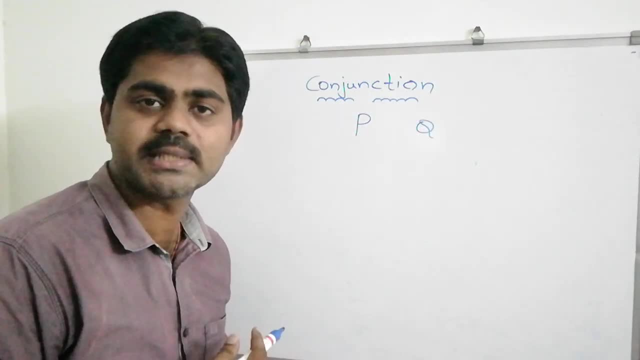 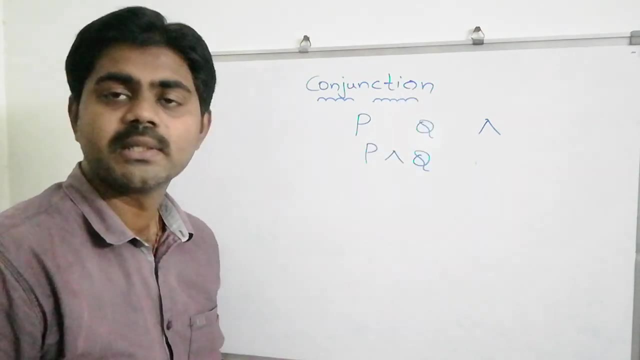 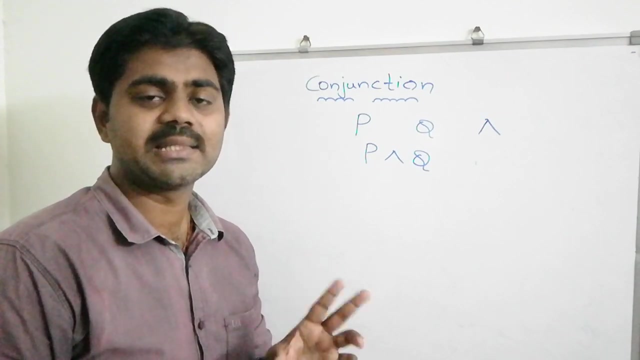 So what is the notation I use here? What is the symbol I use here? This one, So P and Q. So this one is conjunction. So how your truth table is applicable here. The output is true only when both P and Q are true. 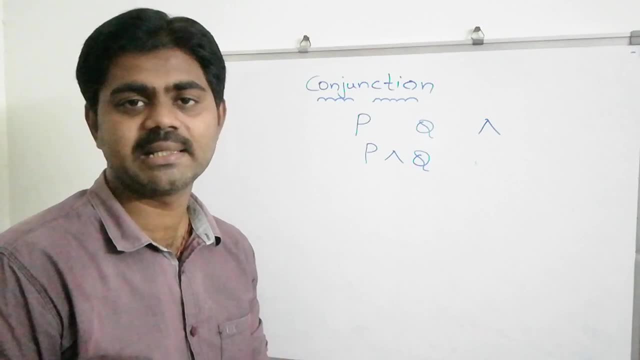 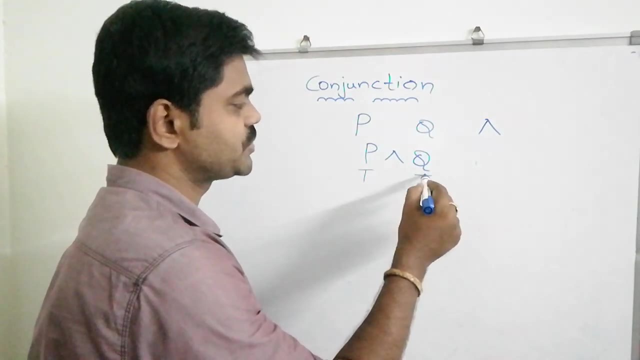 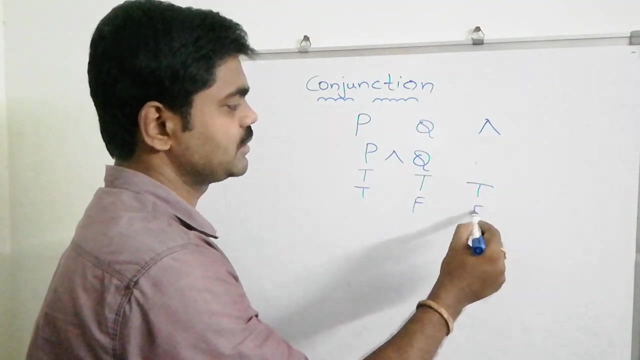 If any one, If any one of the statement is false, then it doesn't hold and the output is false. For example, if P is true and Q is true, then we get result true. If P is true and Q is false, we get false. 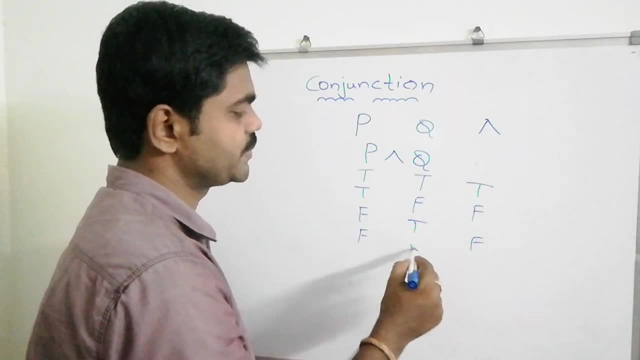 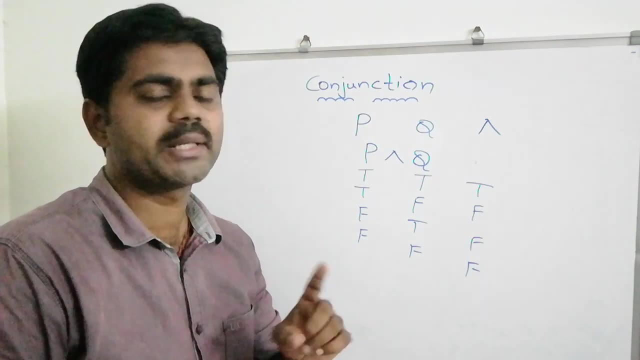 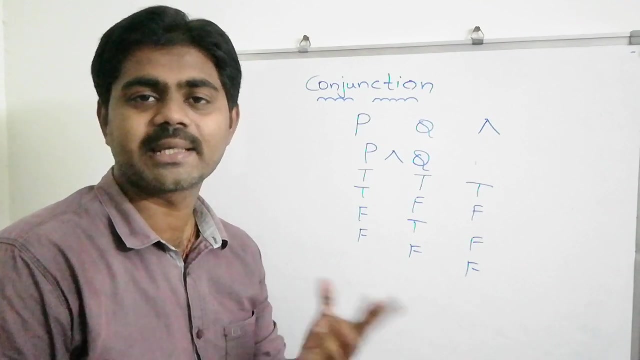 False, true, we get false. False, false, we get false. So what is conjunction here? Conjunction is when P is true and Q is true. If P and Q both holds true, then the output is true In either case, in remaining all cases, the output is false. 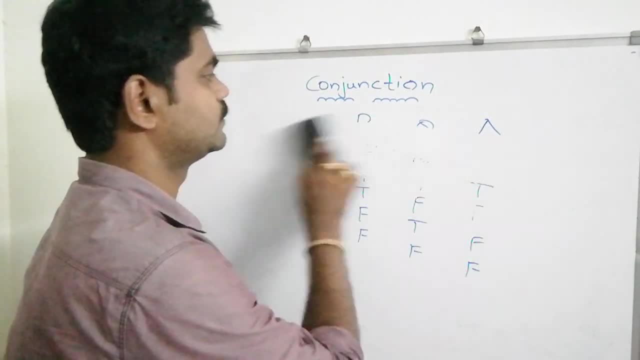 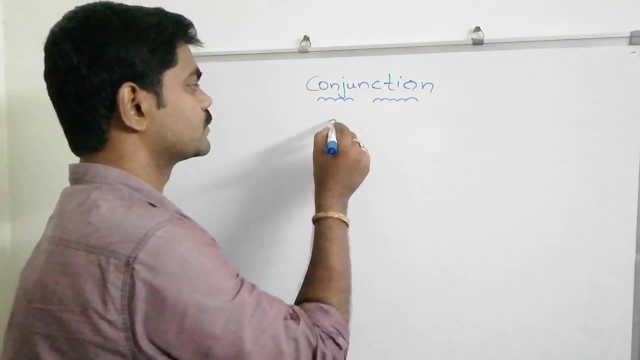 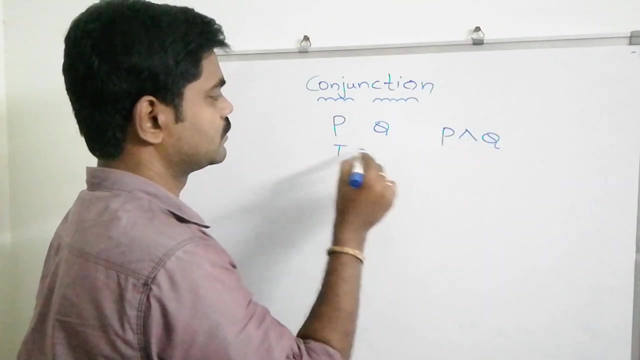 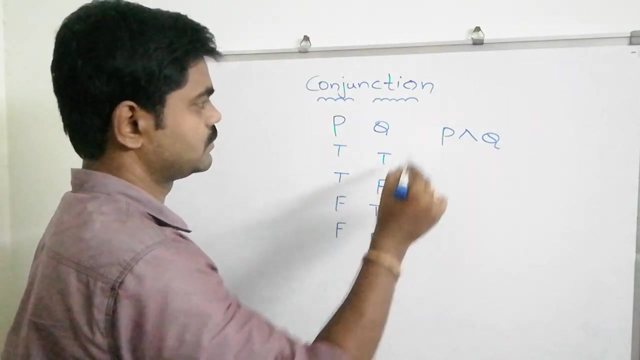 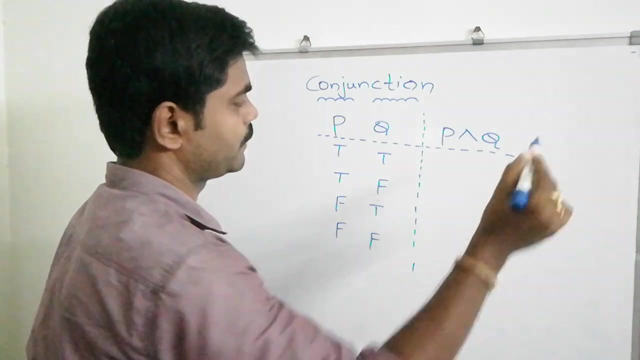 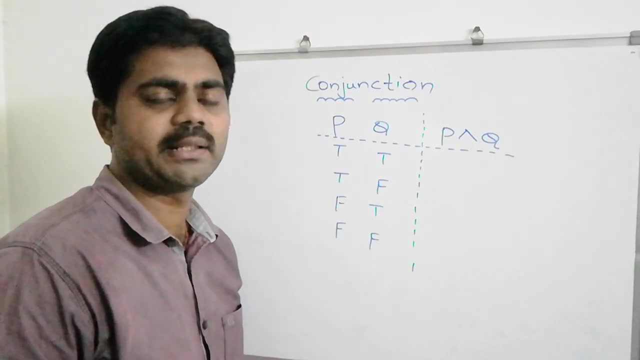 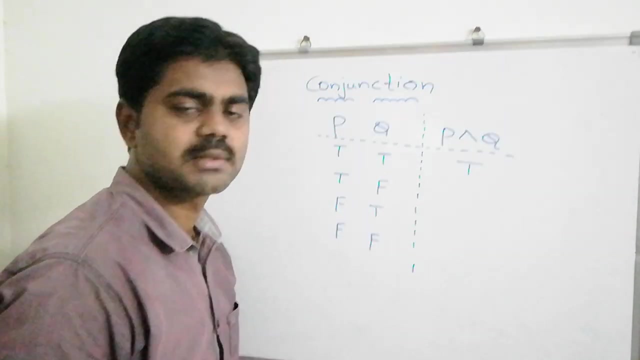 So let us draw a truth table for this. So if we see, here I have P, Q, Here I have true, true for P and Q, Then my output is true, One true and one false, No matter if any one of the statement is false. 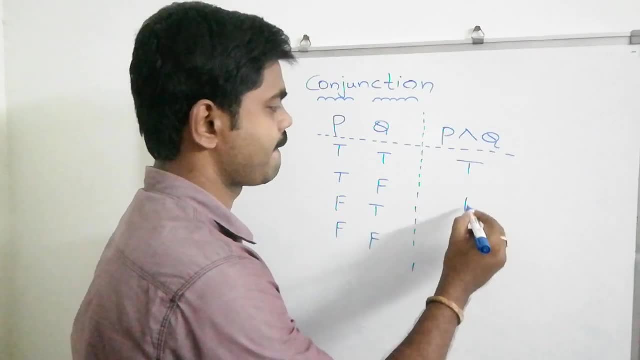 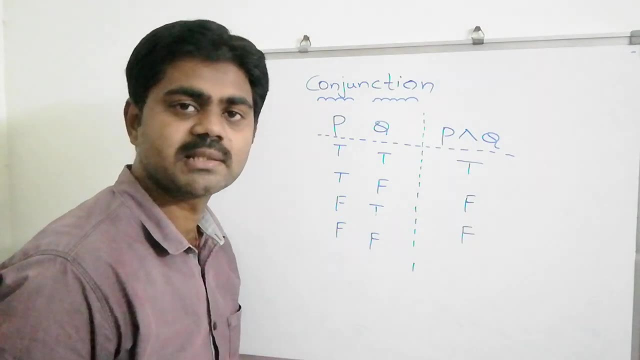 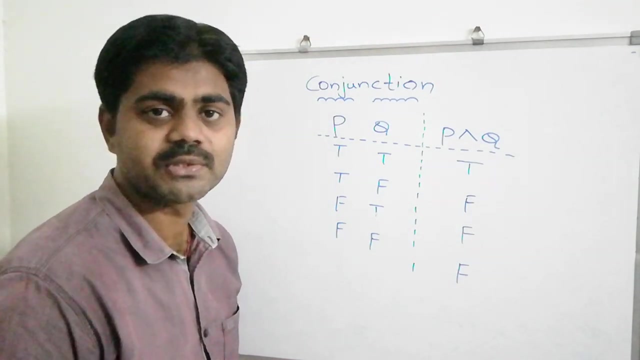 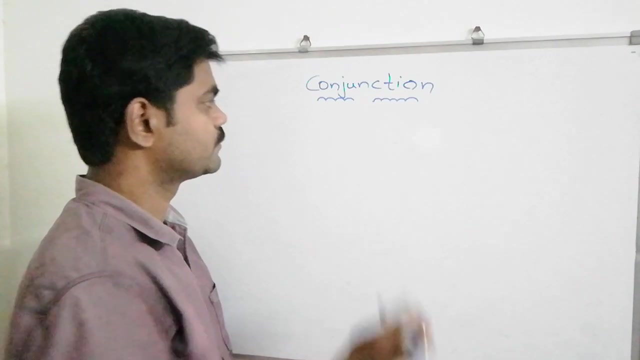 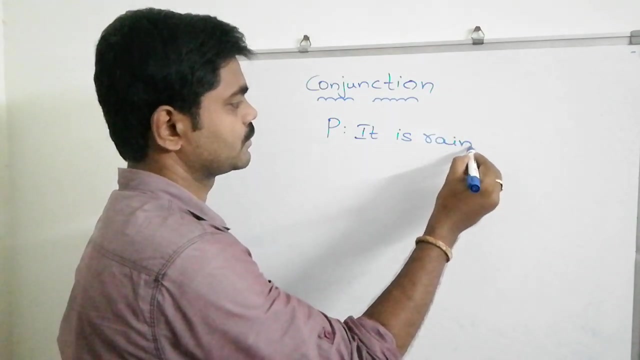 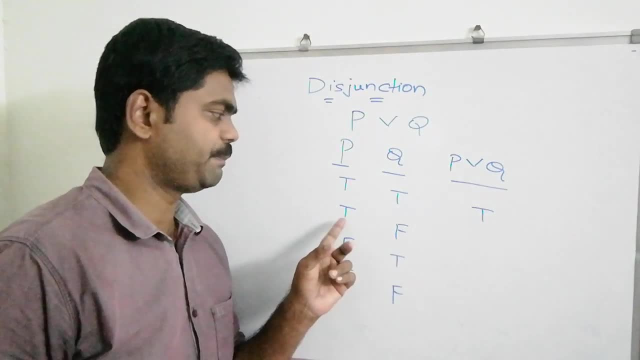 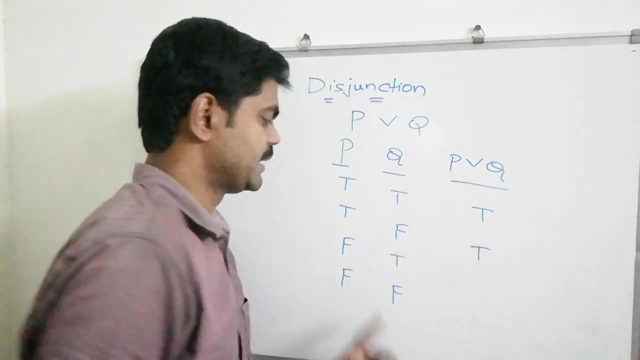 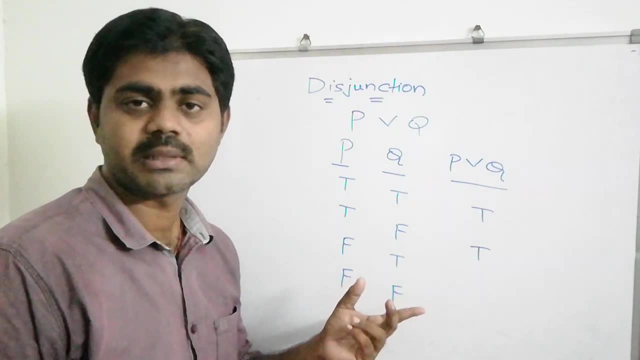 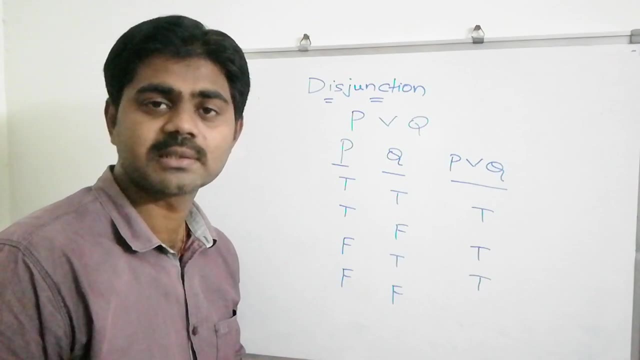 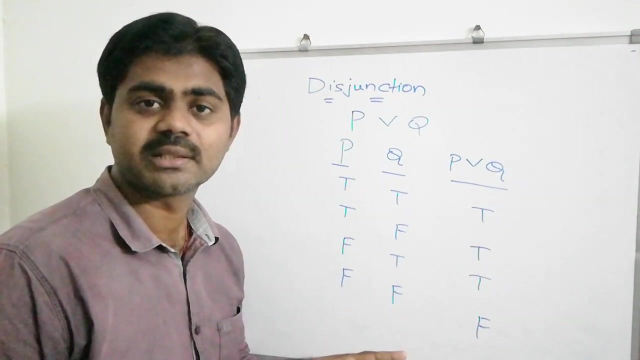 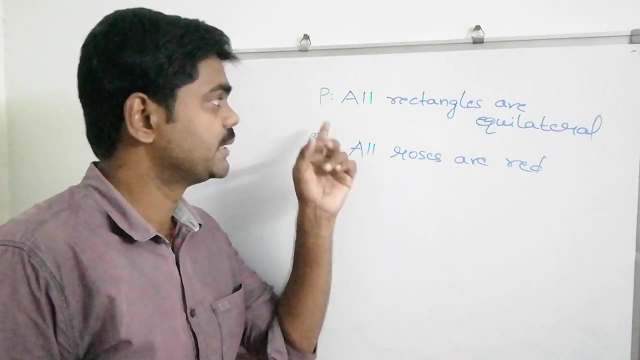 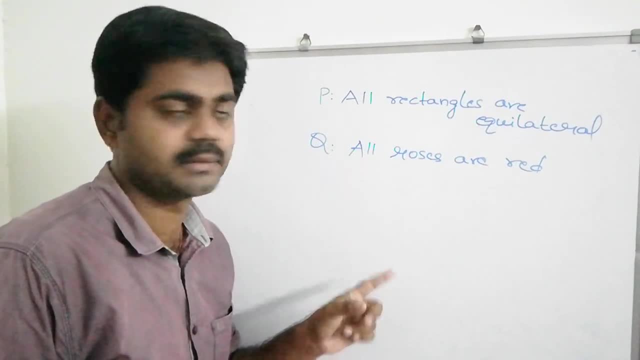 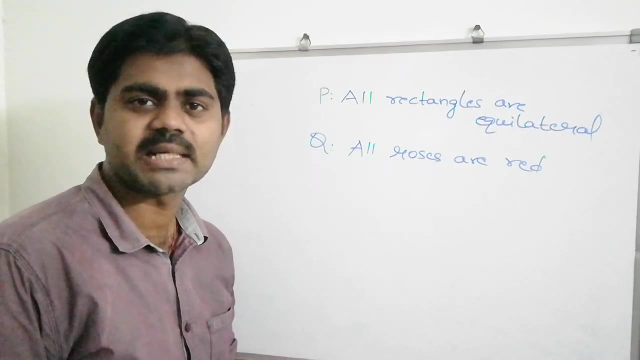 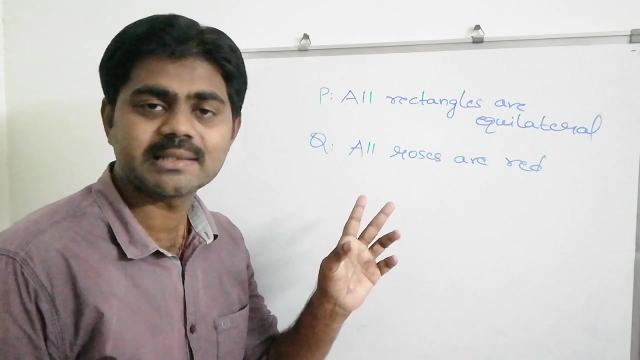 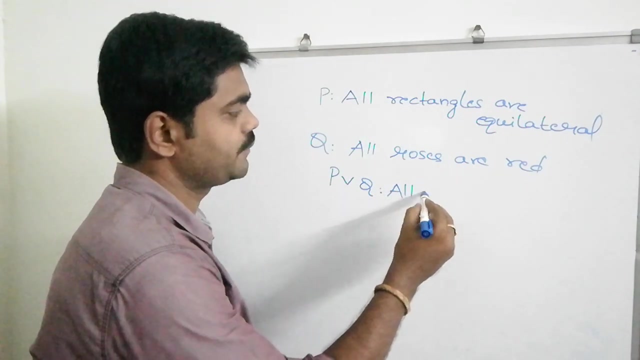 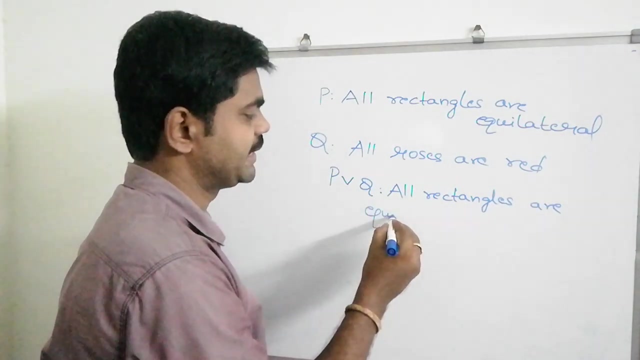 P: all rectangle are equilateral. Q: all roses are red. so if you see Q, there are all roses are red. No, We have white roses, We have yellow roses. Okay, So whatever it is for distinction- P or Q- right? So what can we write? All rectangles are equilateral, or all? 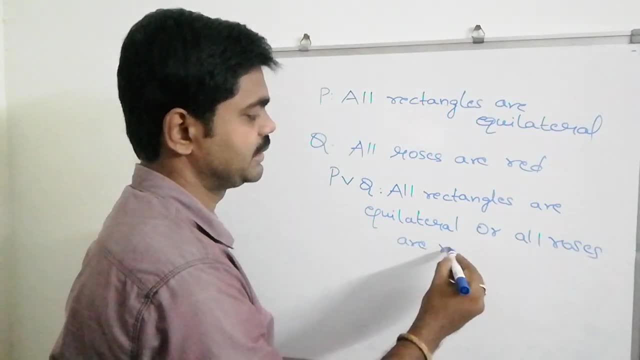 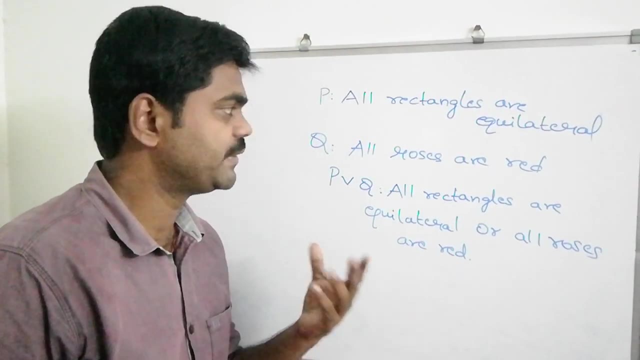 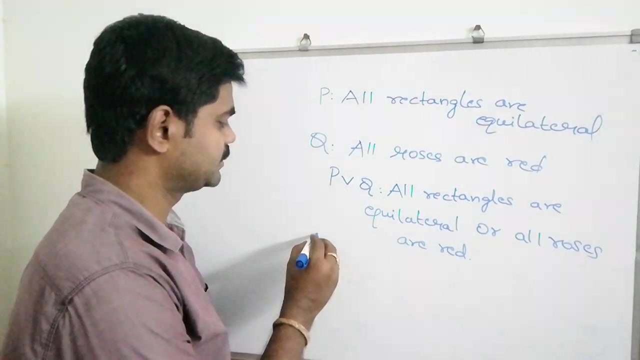 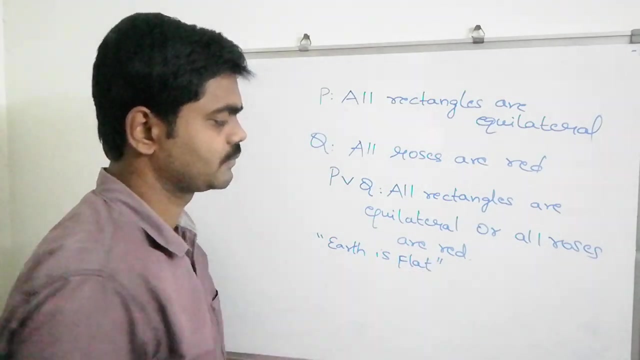 roses are red, All rectangles are equilateral, or all roses are red, So whatever it is for. So, if you take another example, so here we need to obtain a truth value. First one yet is flat Second one: 2 plus 3 equal to 5..